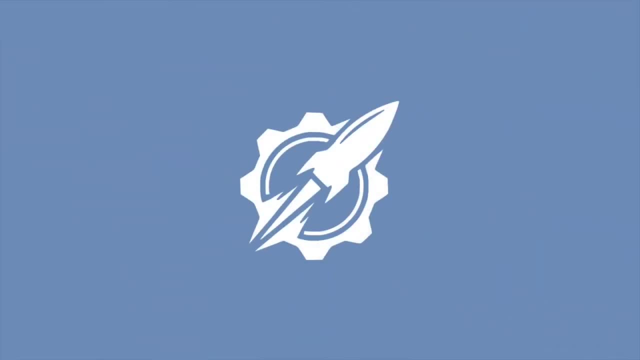 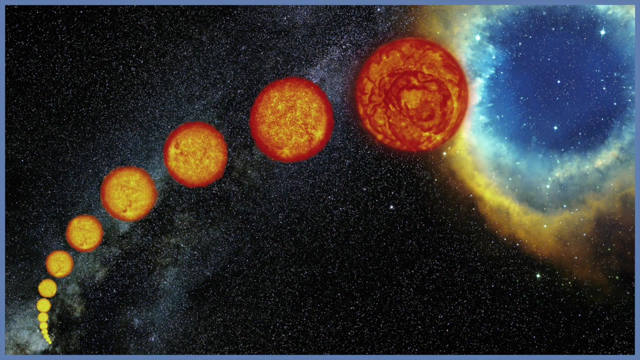 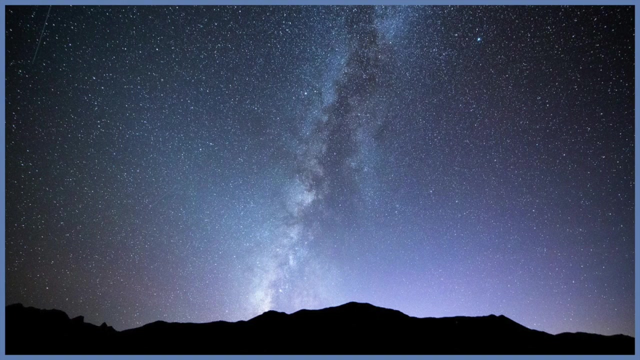 Hello everyone and welcome to our universe. Today we'll be talking about the lifetime of a star. When we look up at the night sky, the stars never really seem to change. In fact, throughout your lifetime, the stars may never change whatsoever, Night after night. 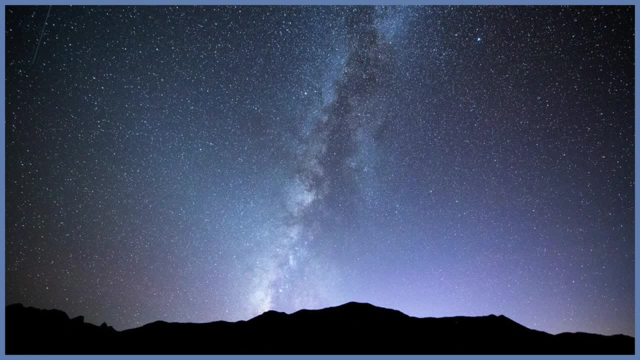 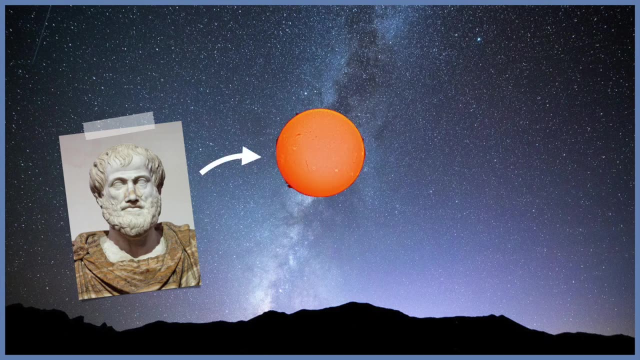 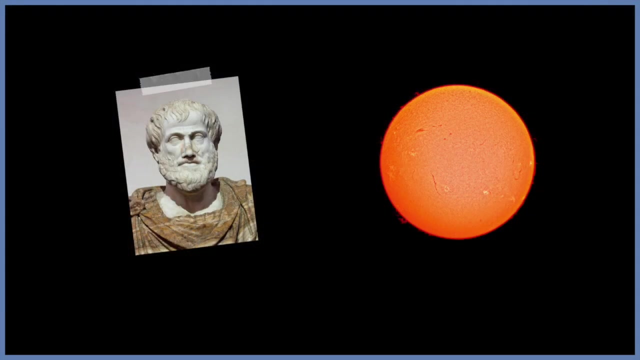 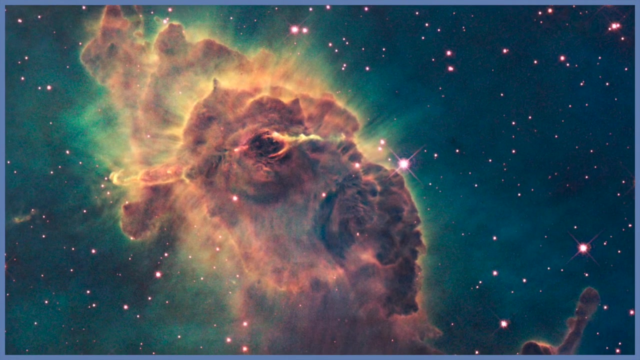 century after century. so many people have assumed through history that they have lasted forever. The Greek philosopher Aristotle even proposed that stars were made of special elements not found on earth. Since Aristotle's time, astronomers have discovered that stars, like people, have finite lifetimes. Stars are born from great reservoirs of cosmic material. 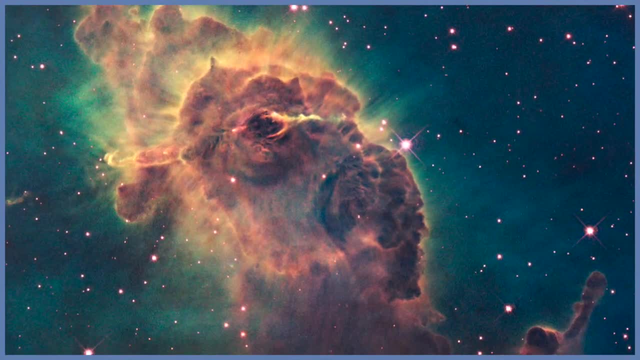 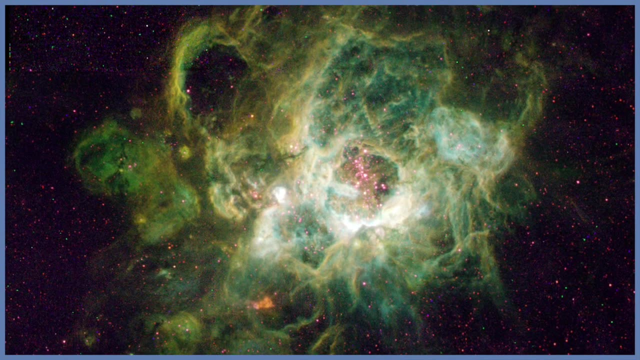 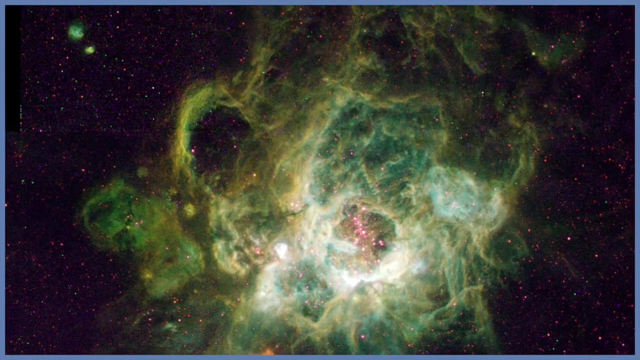 and these are the most common elements in the universe. They shine with immense brightness and give off so much energy for millions, if not billions, of years. However, stars do exhaust their energy supply and eventually die down and go extinct. Understanding the lifetime of a star has been one of the greatest tasks in astronomy. 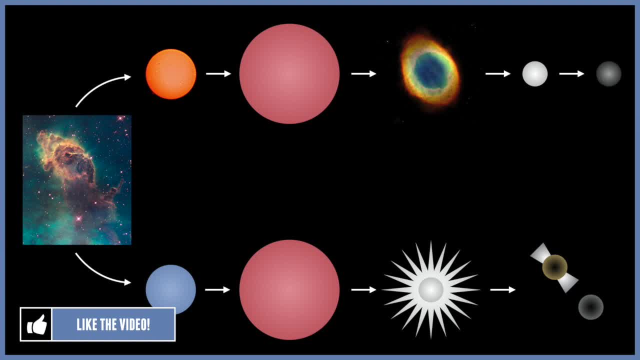 at least during the last hundred years, Astronomers have made remarkable progress in tracking the progression of the stages of a star's phase. So let's review the broad outlines of a star's story and how an astronomical object can be assessed in a sort of lifetime from birth to death, and understanding every stage that a star usually goes through. 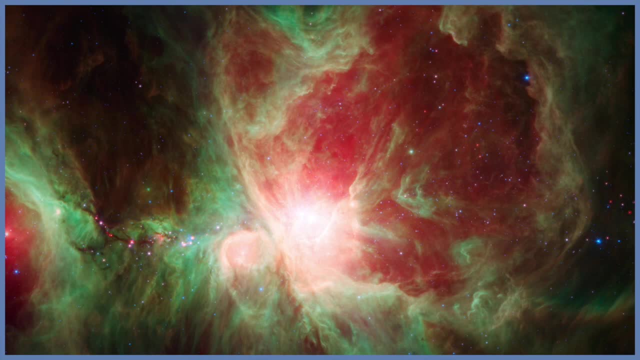 So a star begins their life in a kind of incubation. When a dense region happens to form from a huge cloud of dust and gas, the material that will make up the star falls inwards under the influence of gravity, As the clump of star stuff gets more and more compressed. 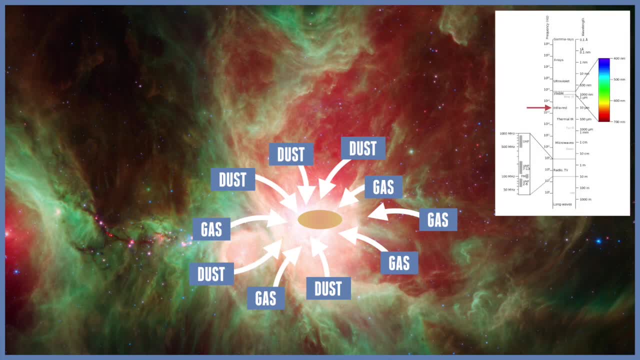 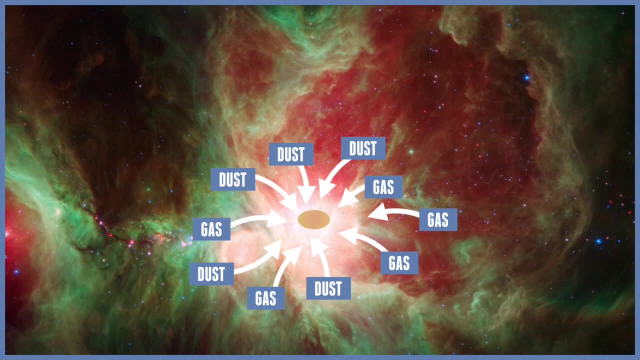 it heats up First with infrared energy and then through visible light. As gravity continues to pull the infant star together, the centre of the collapsing ball of gas gets hotter and hotter, until temperatures at the middle reach an astonishing 10 billion degrees Celsius. 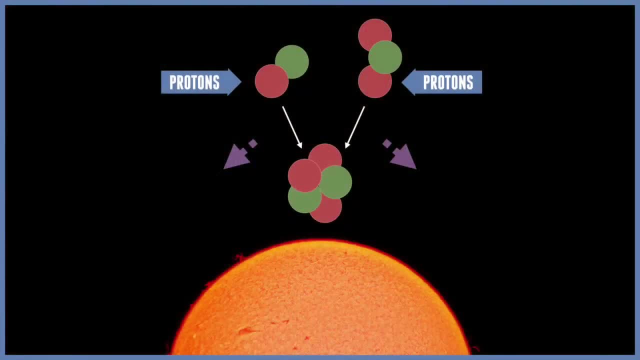 At this temperature, protons can collide so forcefully that nuclear fusion can occur. Physicists call this reaction fusion, because protons that are released into the atmosphere are called protons. because protons that are released into the atmosphere are called protons. Photons are formed originally in the nucleus, fused together to make the nuclei of heavier atom. In a star like our Sun, 4 atoms of hydrogen eventually combine via fusion to make a heavier nucleus of helium Photon. make a lot of backije. photon can still be formed and present within the atmosphere. Death forms a lot stronger, but that's causelated by federation and winds. What makes fusion inside of a star so useful is the transformation of the element, making it into a slightly heavier one, and this releases energy. 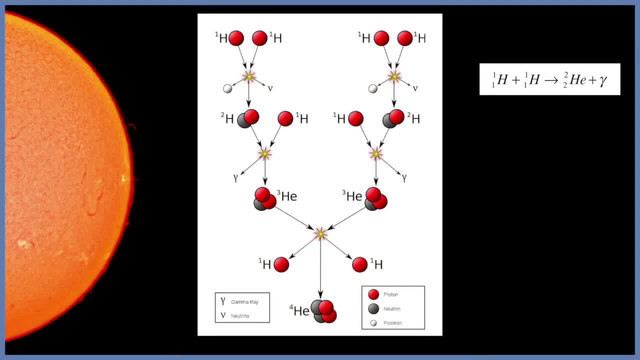 causahlium, which has become fusing in a star beautiful element, is basically a Energie-Soul fusion. Hepatigen and two other 2005 link added by the stream seem to help achieve this Hepicird's Fusion. see the binary composition. 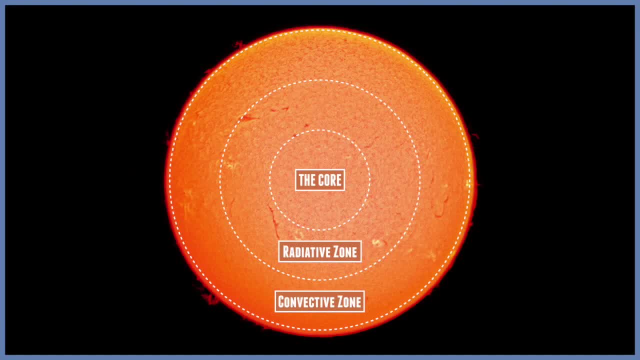 When both are required for the fusion process. topies are created in a mac Statachmi. the mixture remains spinning about other ancient ones. fusion reactions flows outward from the star's core. Some of it eventually emerges from the star's surface as light, The pressure of sunlight, along with particles blown off. 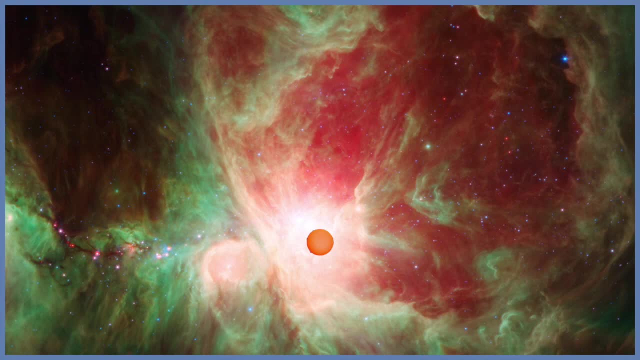 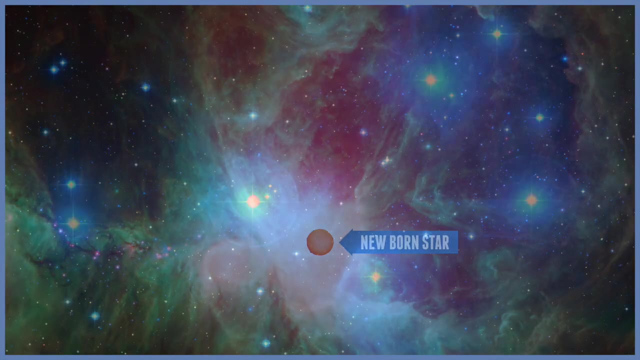 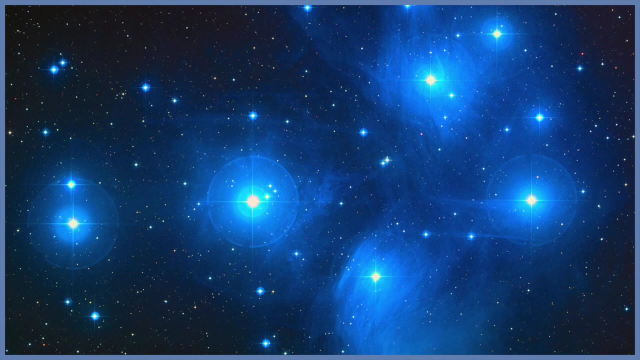 the surface of the newborn star sweep away from the surrounding cloud of gas and dust, and therefore a star is now born. Most stars are born in groups. these are often called star clusters. Clusters like this that stay together allow us to track the stories. 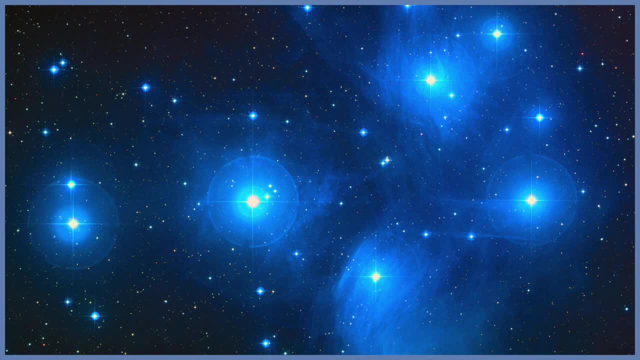 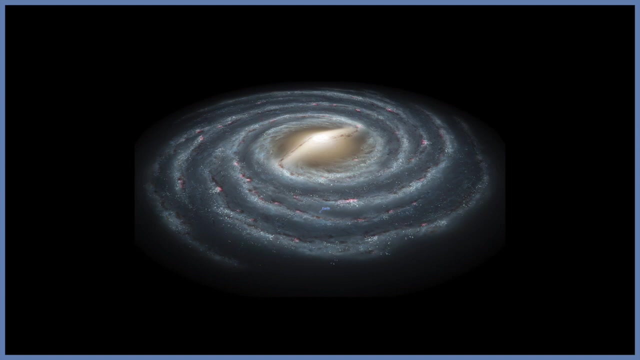 of the stars, while less massive clusters will simply dissolve because of the lack of gravity. These stars in less massive clusters will eventually mix into the general population of the Milky Way. Most stars will simply wander the galaxy until they get into a stable orbit. 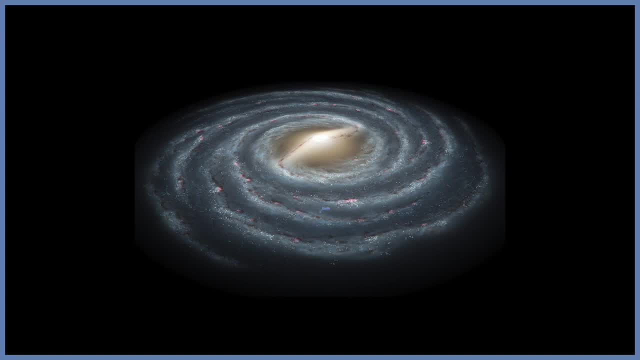 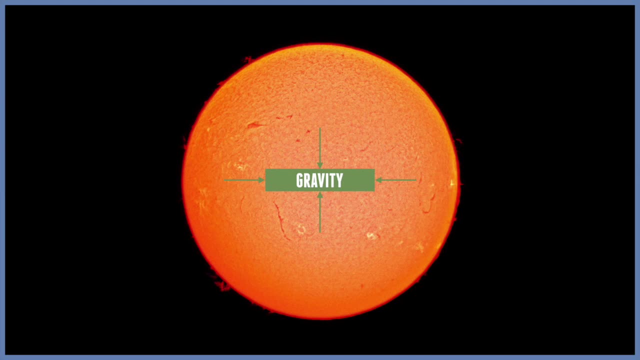 very similar to how a planet orbits a star. The outward push from nuclear fusion in its core is now nicely balanced with the inward push of gravity, and the star remains in this balanced state for about 90% of its lifetime. This is now at the stage that the sun is now in. It's been at this stage for almost 5. 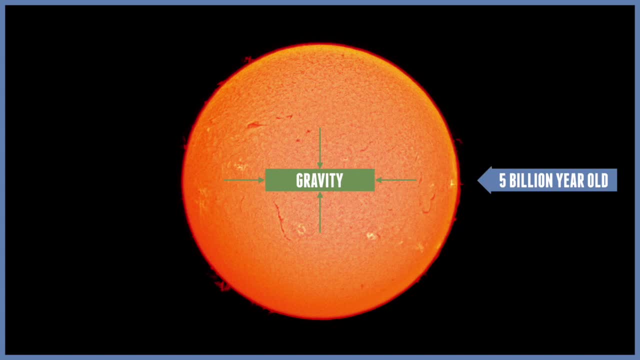 billion years, and it will continue to do this for at least another 5 billion years more. Having a stable star is thought to be critical to the development and evolution of life, and how long a star lives depends on how much material or mass it has. 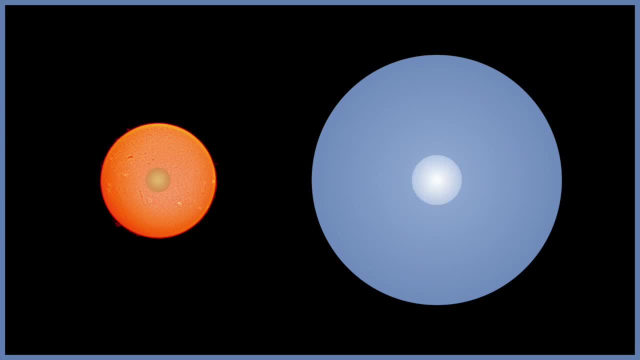 Massive stars have a lot of gravity, which makes their centres extremely hot and therefore they tear through their hydrogen atoms extremely fast and exhaust their fuel very quickly. The most massive known stars last only a few million years. The core of the lower mass 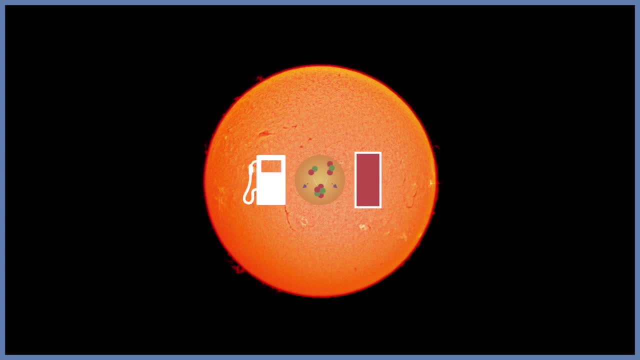 stars, like our sun, is almost impossible to measure and the atmosphere is almost impossible to measure, lot less hot and burns its fuel a lot more slowly. this means that our star can last for billions of years rather than just millions. the lowest mass stars, known as the dwarf stars, burn very, very. 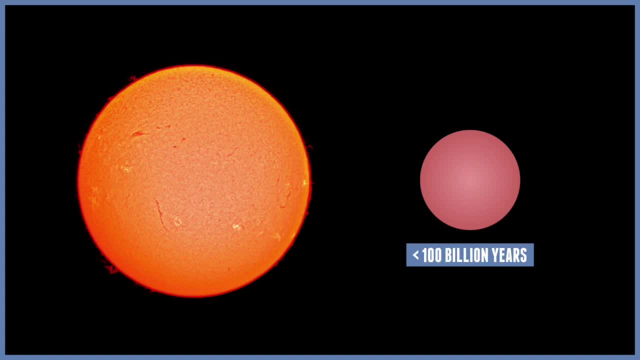 slowly and they may last more than a hundred billion years. this is much longer than even the current age of our universe. nevertheless, the core of every star eventually runs low on nuclear fuel. at this point, the star experiences a bit of a crisis. gravity is still compressing. 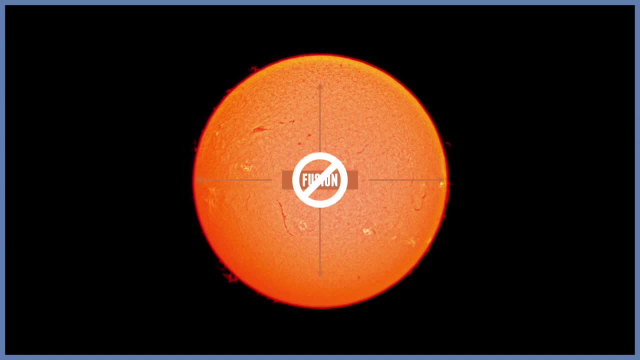 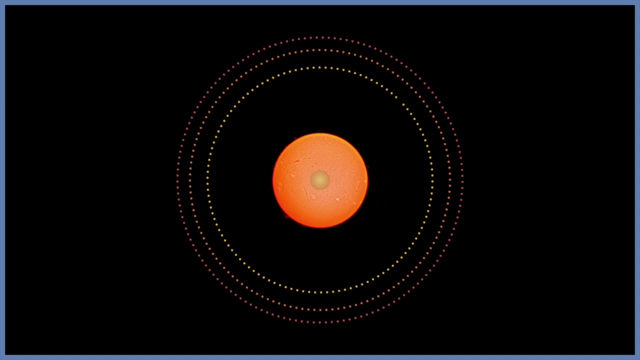 the star, but the outward push of fusion begins to suffer. a complex series of vents then occurs, which leads the star to collapse on the inside whilst it swells up on the outside. as the outer layers of the star grow larger, they cool off and become reddish in color. a red star is. cool enough to completely crumble down the entire subspace, which means that our stars is very much more springy. I figured that would be something about, okay, um, if the dense and moist transport so well work our weather. imagine if gelen washn going on like a giant бел. imageries were to be a myriad. but 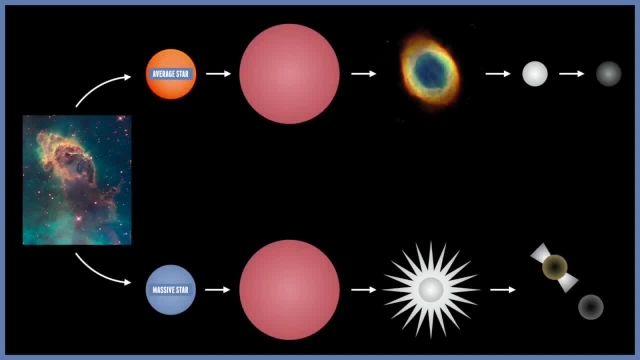 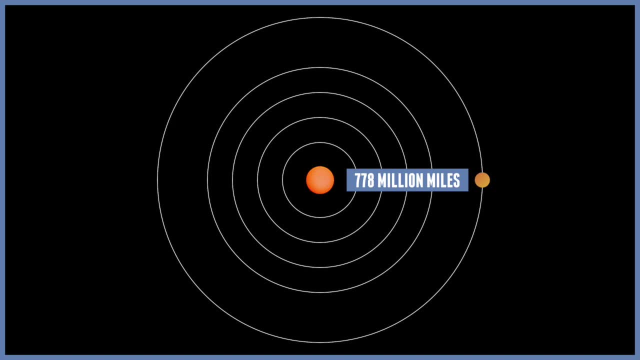 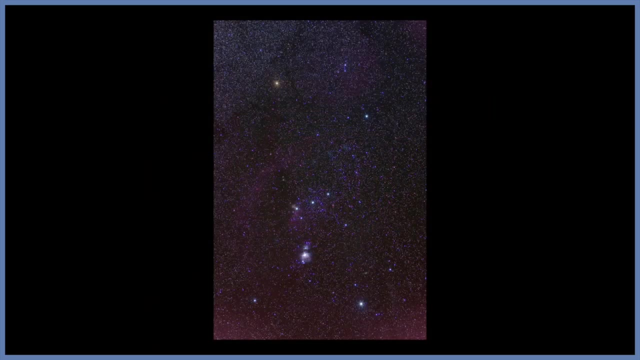 at its surface than a white star. Astronomers call these type of stars red giants, and they can become as large as the orbit of Mars or even Jupiter. A particularly dramatic example of a red giant is the star Betelgeuse: It is 425. 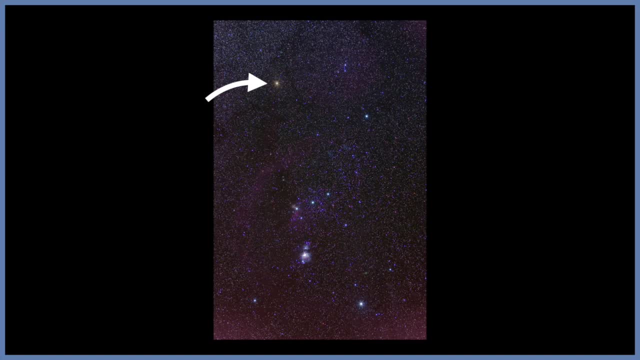 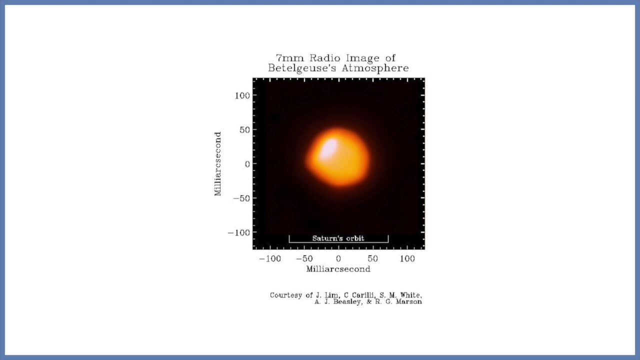 light-years away from Earth in the constellation of Orion, so it's astronomically quite close. It has now grown to be 600 times larger than our Sun and would it to replace our Sun at the center of the Sol system, it would completely swallow the orbits of all of the inner planets, But all red giants. 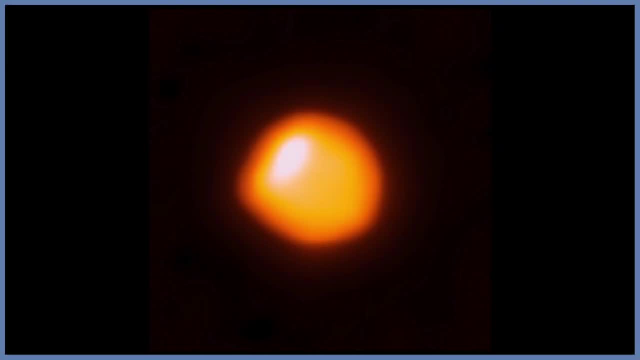 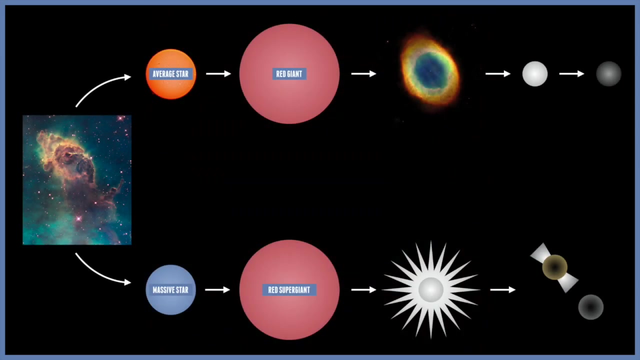 eventually do find a new source of fuel, But the star is never quite the same again. Some of its outer layers are permanently lost and it's resumed instability is only temporary. The lifetime of stars splits into two branches. The low-mass stars, which is our Sun, have 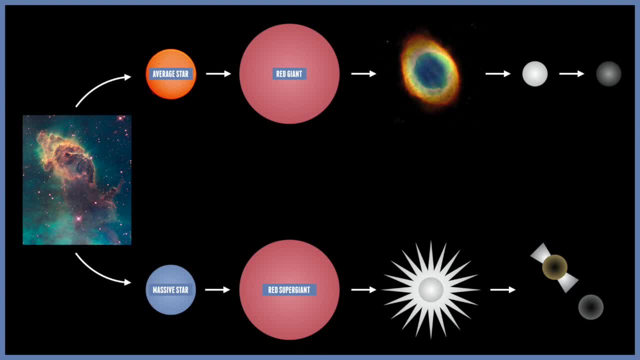 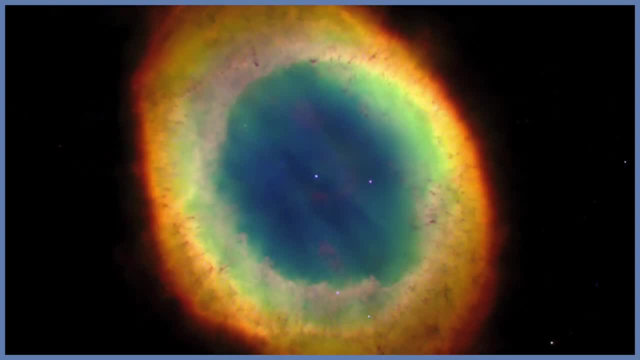 only a little bit of space between them and a little bit of space between them. They have a limited ability to squeeze their cores to continue the fusion processes. They experience a period of instability where their outer layers lift off. This period of instability for those stars produce some of the most 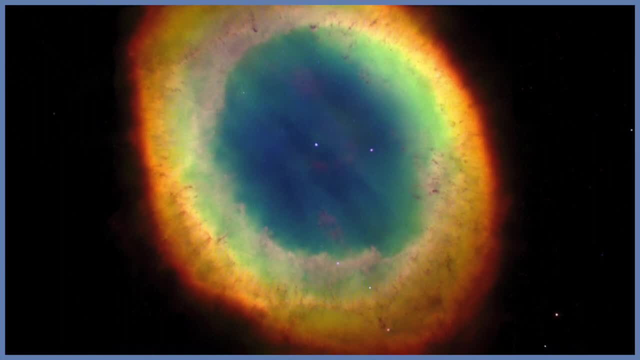 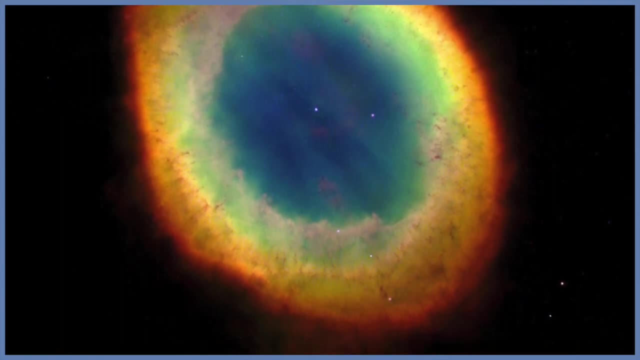 beautiful objects in the night sky. As a star shreds its outer layers, the gas inside of it is illuminated by the light of the collapsing star and glows in an array of colors. These are the last gasps of a dying star. 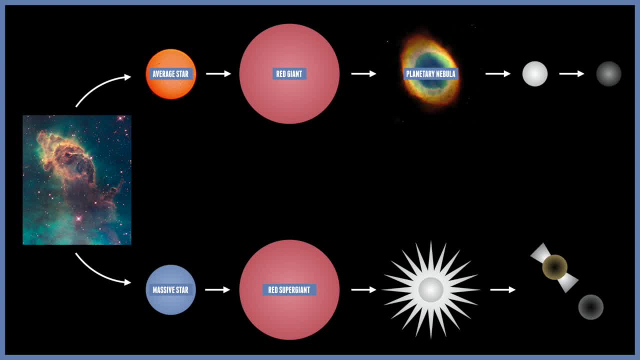 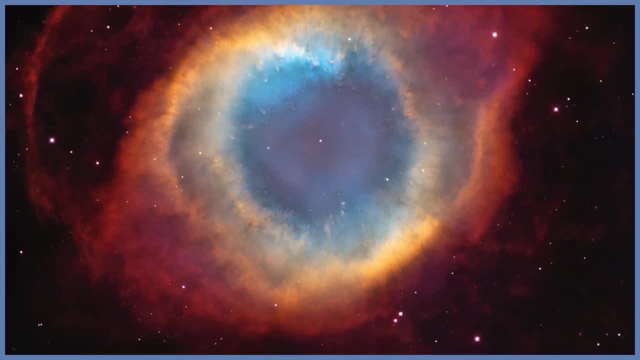 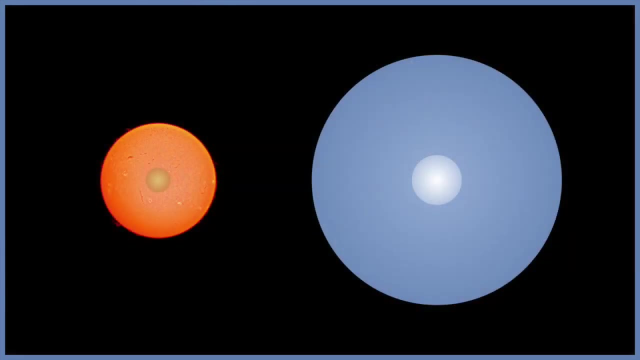 These objects were named planetary nebulae because they resemble disks of planets, although we now understand that they have no connection at all to planets, But the name, of course, has stuck. So, on the other hand, high-mass stars have significant pressure and temperature at their cores, and this means 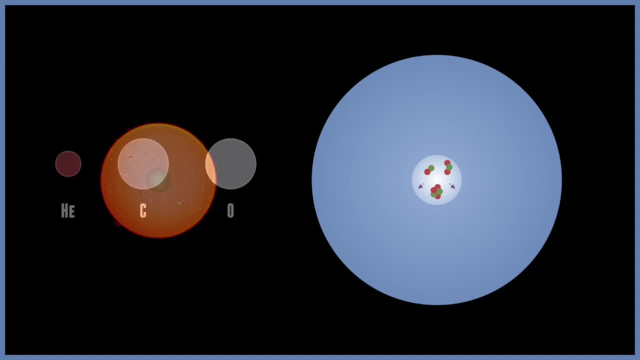 that they can continue the fusing process by using these newer, heavier atoms that they formed earlier: Helium carbonate and carbonate. They are all in turn becoming fuel to make more energy for the star, and this is fighting against the gravity And this keeps the star stable, at least for a brief time. 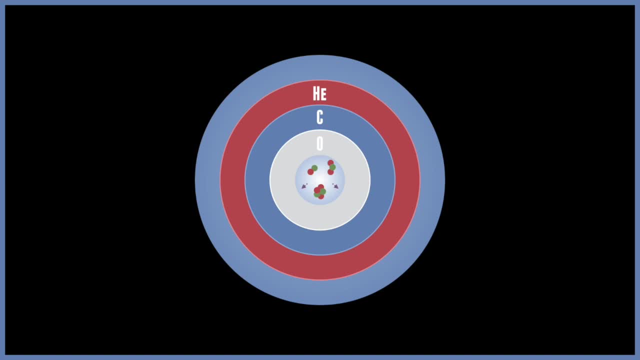 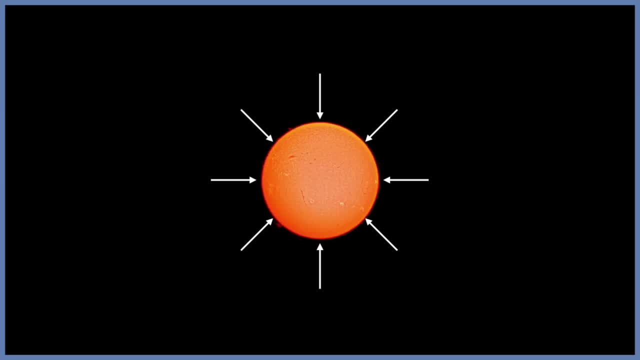 When low-mass stars die, they collapse under their own wells. Until their centers act in the same ways, like a solid, A star like our Sun will collapse at the end of about twice the size of Earth. These white, hot dying stars are called white dwarfs by astronomers. Perhaps the 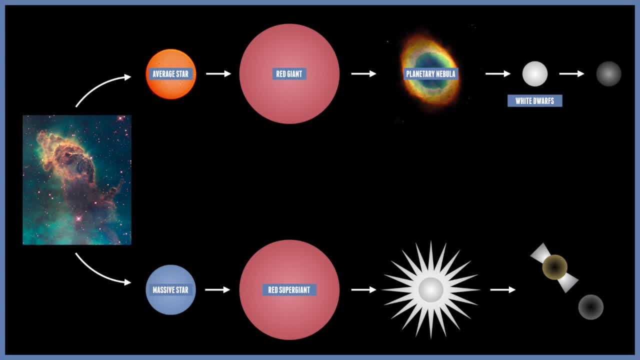 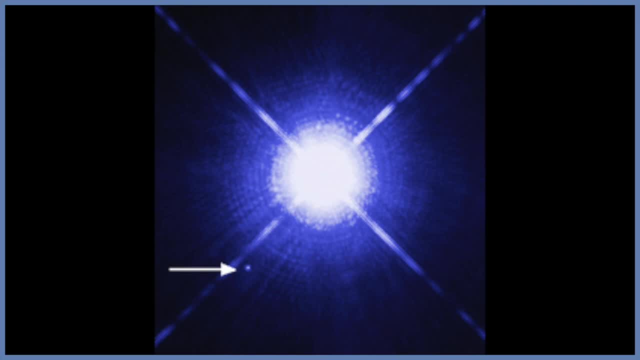 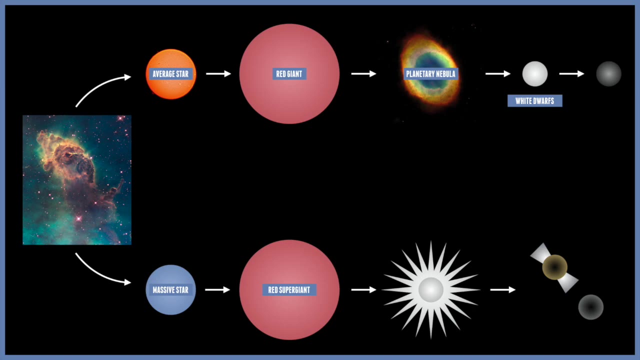 best-known white dwarf orbits the brightest star in the sky. Serious, But it requires quite a large telescope to see it. Massive stars are very different. in their ending, when the core of a massive star collapses, its powerful gravity takes it right through the white dwarf stage to produce one of two extremely bizarre objects: either a neutron, 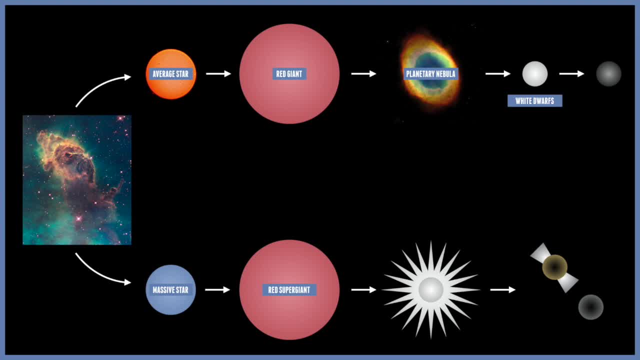 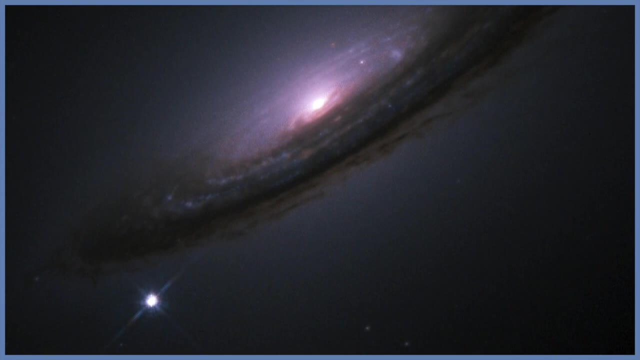 star or a black hole. in most cases, the rest of the star blows up in a gargantuan explosion called a supernova. these explosions produce so much energy that the star can briefly become brighter than the entire galaxy in which it's located. this is approximately brighter than 100. 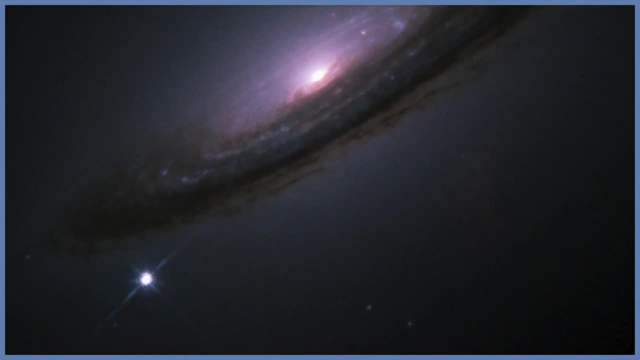 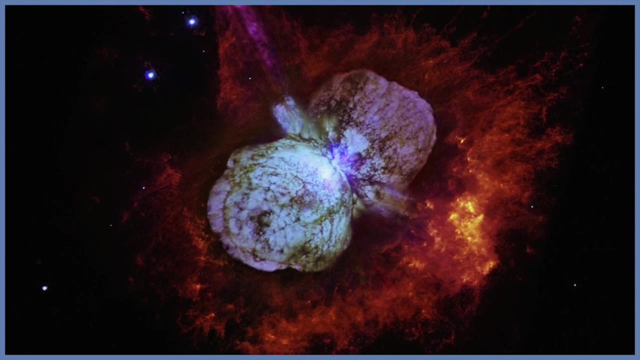 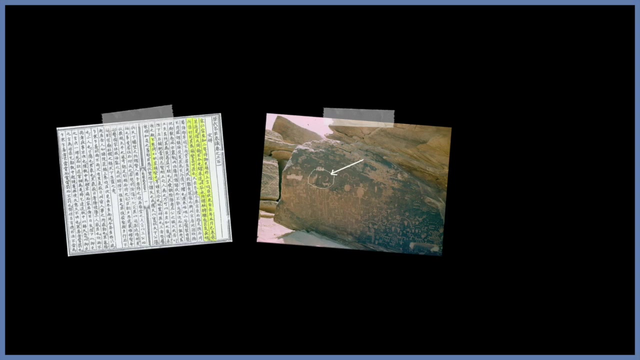 billion suns. extreme versions of supernova explosions are sometimes referred to as hypernovae, and these produce gamma-ray bursts. the most famous supernova in history was in july 1054. records of this still survive from china all the way to north america, seen today. 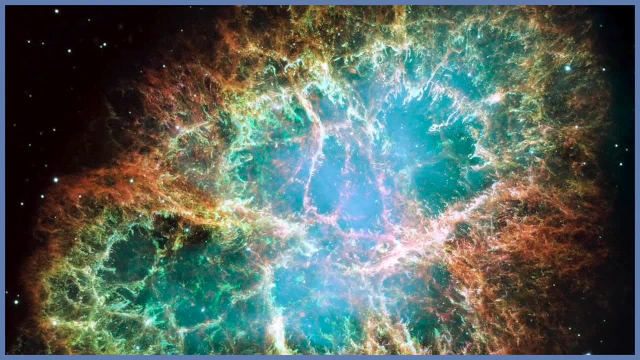 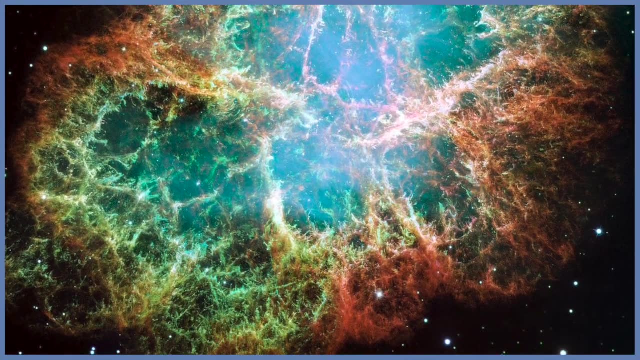 roughly a thousand years ago, the supernova was the largest supernova in the world and years later its remnant is called the crab nebula and is one of the most interesting objects in the night sky. it can be found with a good pair of binoculars or a small telescope in the constellation. 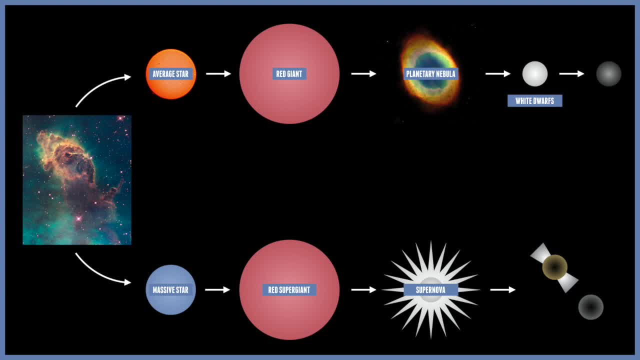 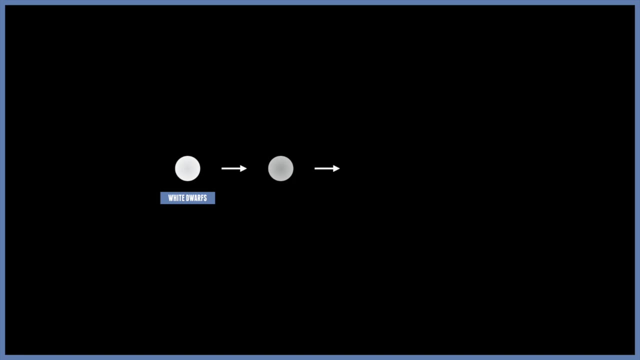 of taurus near enough. every star leaves a corpse. star corpses come in three bizarre varieties. a white dwarf fades away as billions of years pass. since no energy is being produced inside of it and is escaping off into space, the star's corpse slowly cools down and becomes black as space. 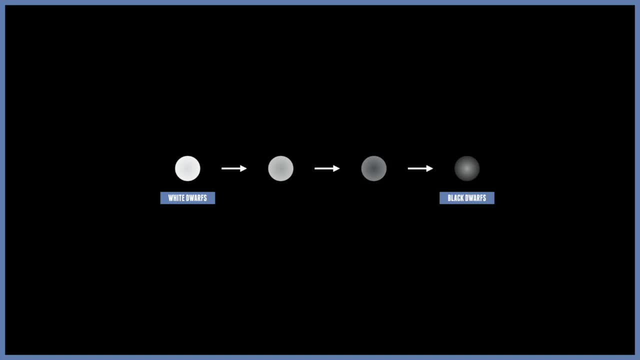 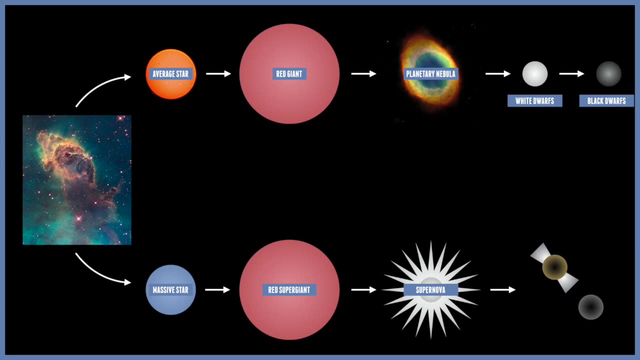 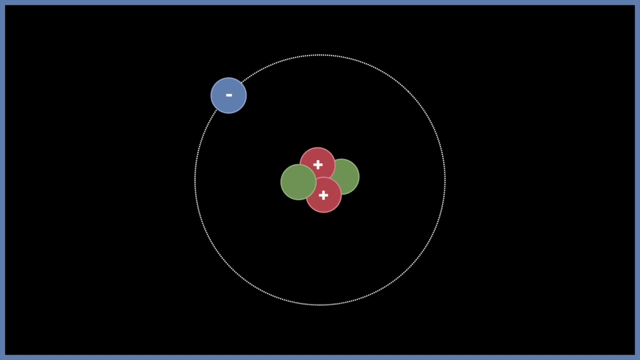 astronomers call these corpses black dwarfs. a supernova explosion leaves behind a far more compressed corpse. the violent end to a massive star produces so much pressure that the star's core experiences a remarkable subatomic change. electrons that are negatively charged particles which orbit the nucleus of the atom, are actually squeezed into the nucleus. the electrons join with. 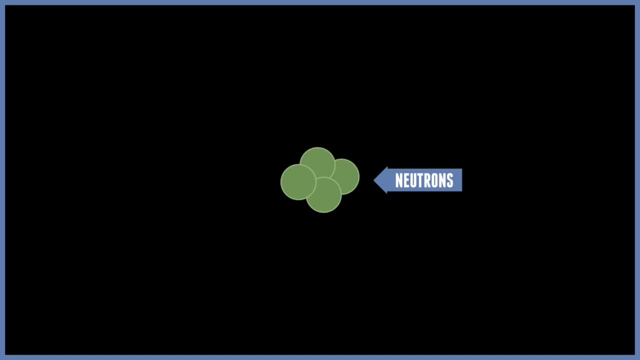 the protons to become neutrons. the process also removes all the space within the atom, leading to a fantastic compression of a star's remnant. to make something as dense as a neutron star on earth, we would have to take all the people in the world and squeeze them into the size of a 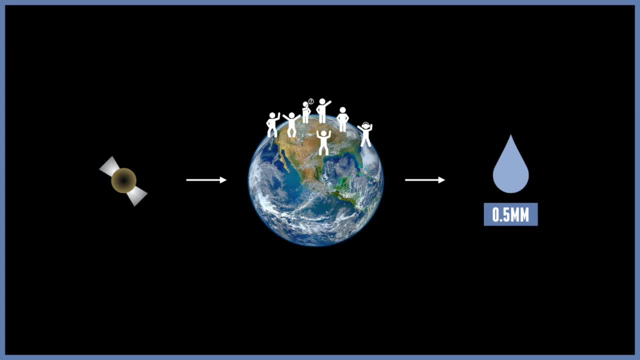 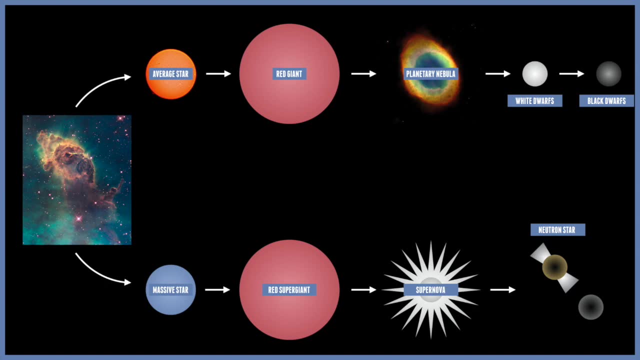 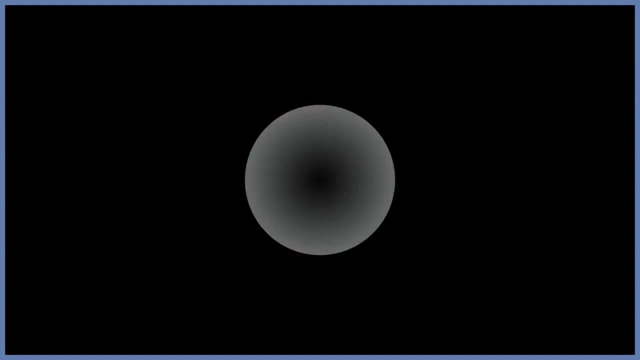 raindrop. if the dying star is especially massive, the remnant becomes a completely collapsed object, known as a black hole. in these objects, gravity is so strong that nothing, not even light, can escape space. time, matter and energy are all trapped within a tiny region. understanding the behavior of black holes is one of the great frontiers in the area of astronomy. 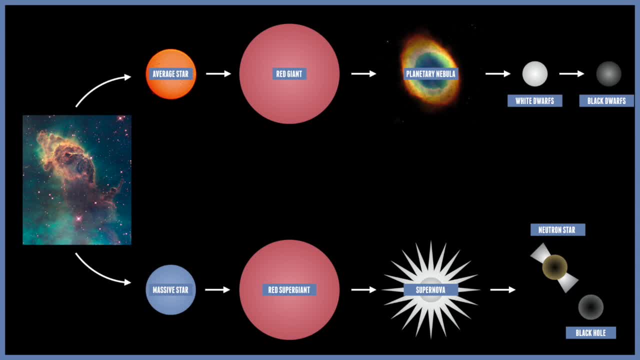 but the reason why we can't see these stars is that this is not a star. it is simply a small part of a star that is ready to be destroyed and is, in fact, a very big part of a human life. so, by looking at a life story of a star, you might be thinking to yourself: how does this interact with? 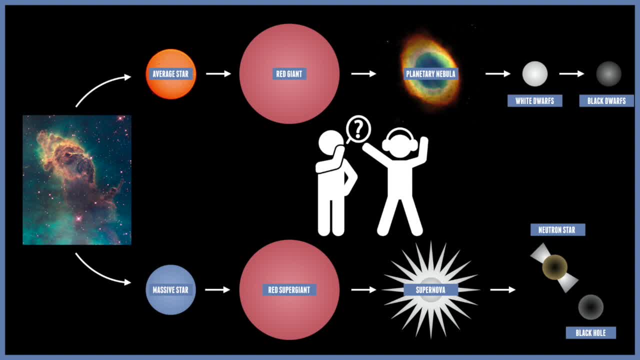 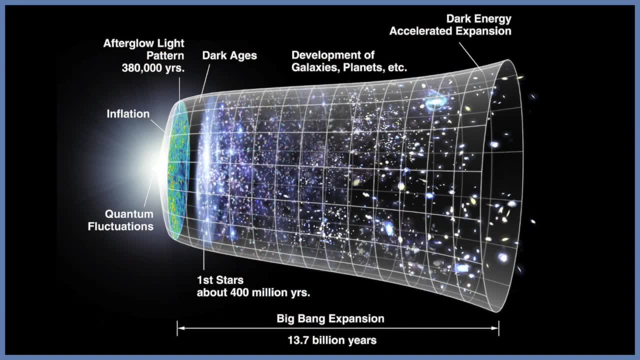 human life here on earth. what's the difference between life and death and previous generations of stars, when it doesn't have anything to really do with humanity? the thing is, stars have a chemical makeup and it all started when the universe began with only the two simplest types of atoms: hydrogen. 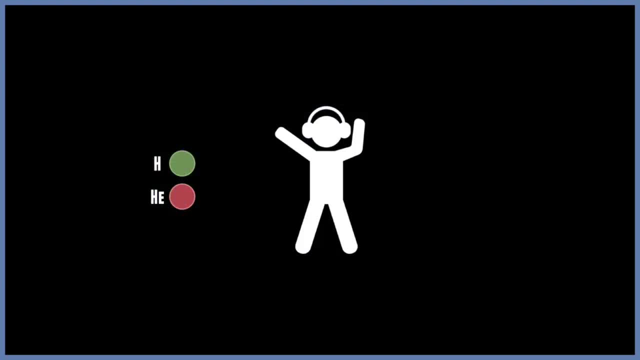 something as complex as a human being out of just these two elements. You need more stuff, so you need things like carbon, oxygen, calcium, iron and a host of other atoms to make a human being, or life in general. So where did these heavier elements come from if they were not present at the start of the universe Well heavier atoms had been produced by nuclear fusion at the centre of stars. We see much evidence that stars create new elements in the process of making energy. When stars die, and especially the ones that go supernova, they seem to recycle their material. 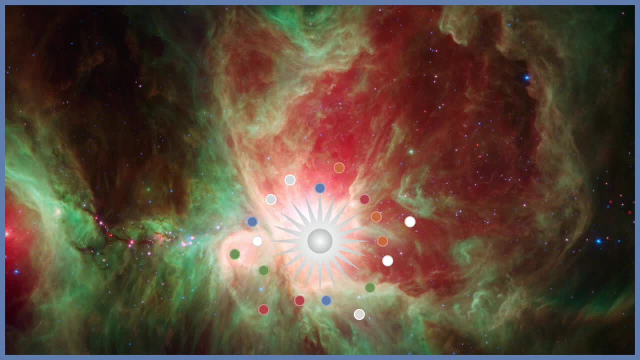 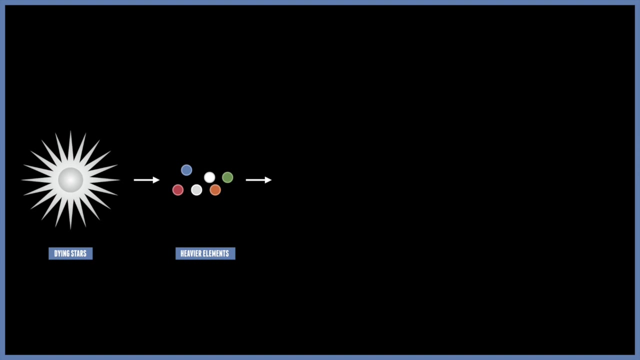 blowing these newly made elements into the cosmos. The next generations of stars then forms from these enriched mixtures of elements, and therefore so do planets. It took several generations of stars to enrich our neighbourhood So that when the sun and the earth were formed 5 billion years ago, they would contain enough. 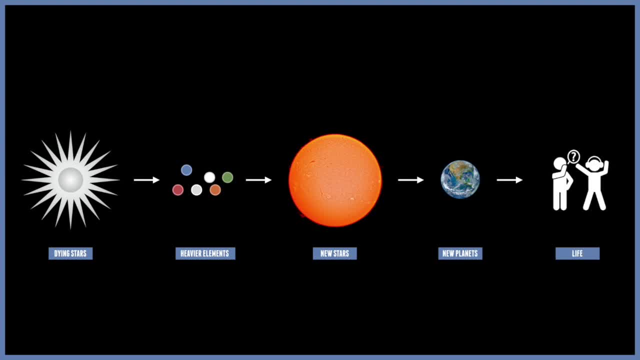 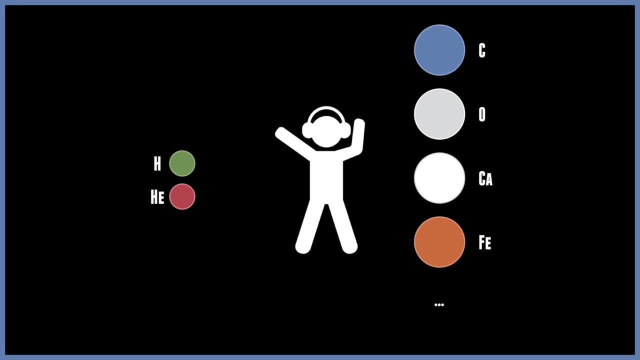 of the heavier atoms to make living creatures. Every atom inside of the human body, apart from hydrogen and helium, of course, was once part of the inside of a massive star, and from this process it can create new life, not only for new stars, not only for new planets, but living organic creatures.